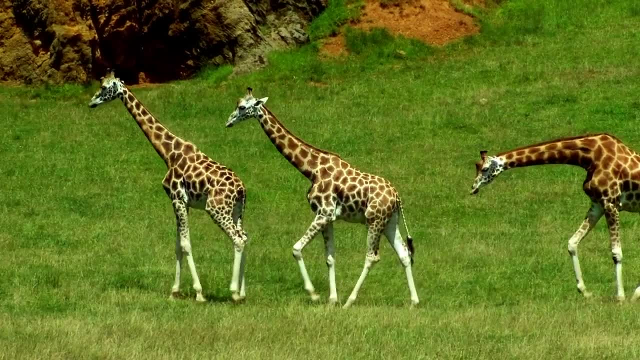 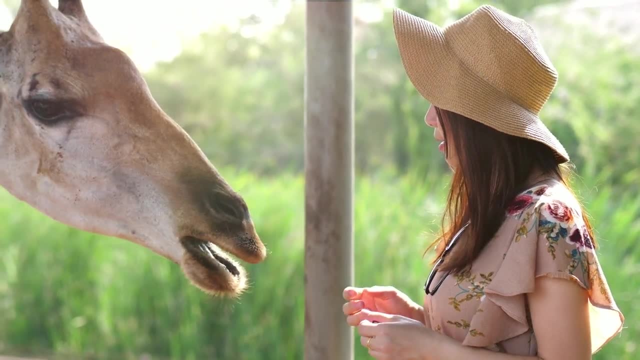 When it comes to the tallest land animal on earth, giraffe is the tallest of all. Due to its height, giraffe always has been the center of attention at zoos and in safari parks. If you have never seen a giraffe, you might wonder: how tall is a giraffe? 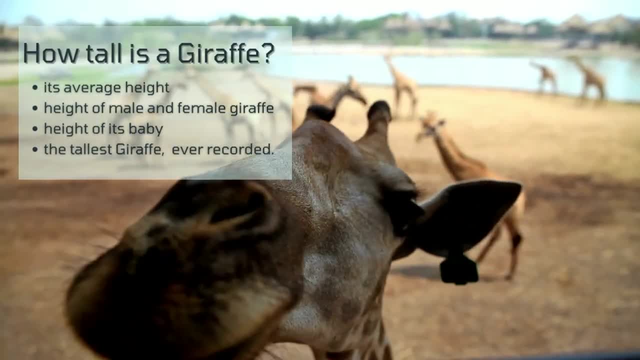 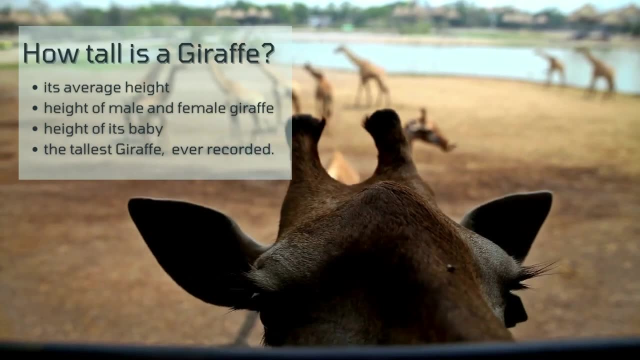 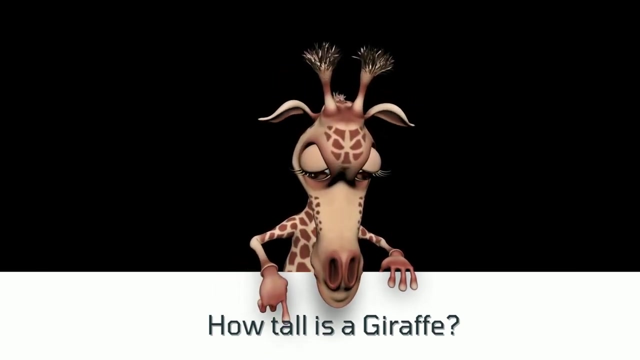 In this video we will discuss the height of giraffe. you will get to know its average height, the individual height of both male and female giraffe, height of its baby and the height of the tallest giraffe ever recorded. When someone asks how tall is a giraffe, it means that the person is asking the average height. 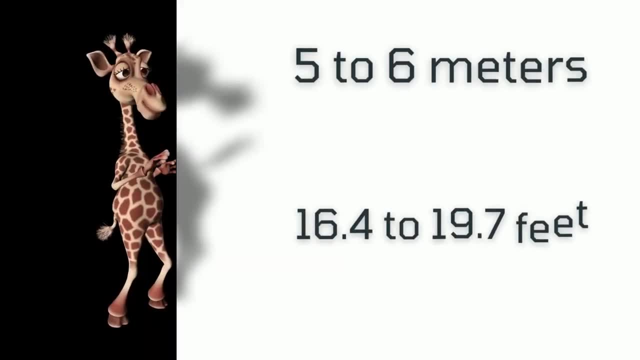 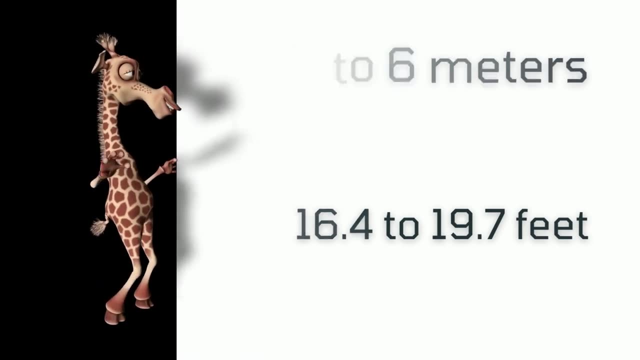 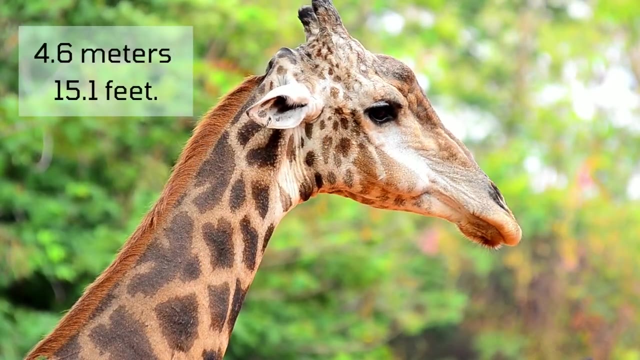 of the adult male giraffe. So the most obvious answer is the average height of the male giraffe, which is five to six meters. The male giraffe is taller than the female giraffe. The average height of a female giraffe is 4.6 meters. 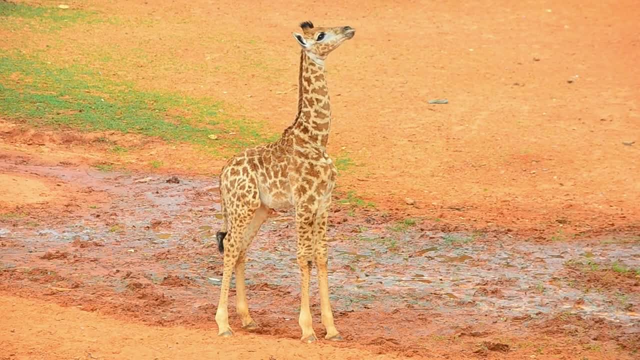 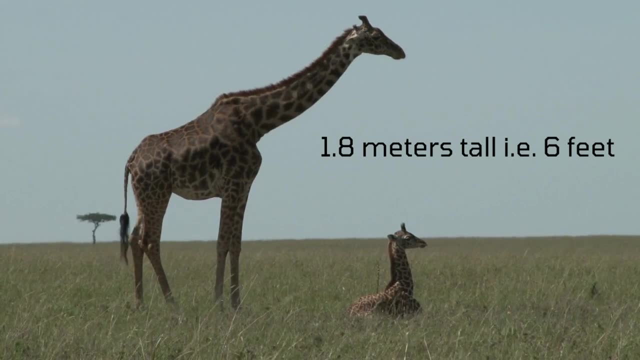 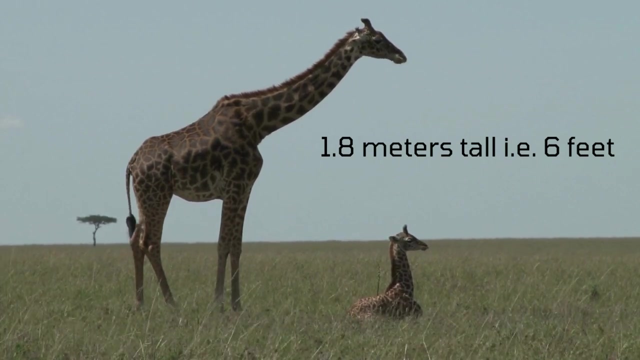 When compared to the babies of other animals, a baby giraffe is the tallest baby at birth among all the animal's babies. A newborn giraffe is about 1.8 meters tall, which is equal to six feet. It is almost the same height as of its mother's legs. 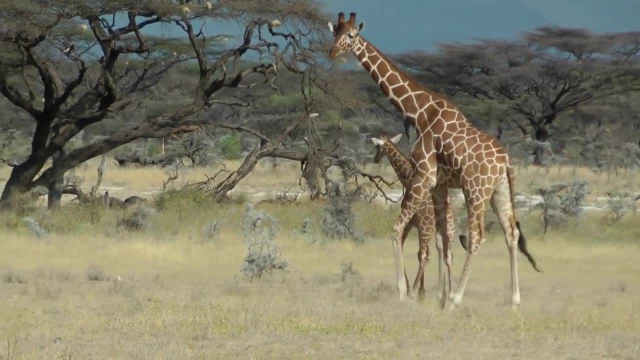 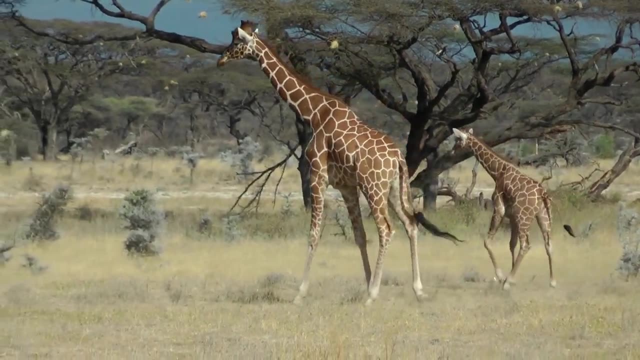 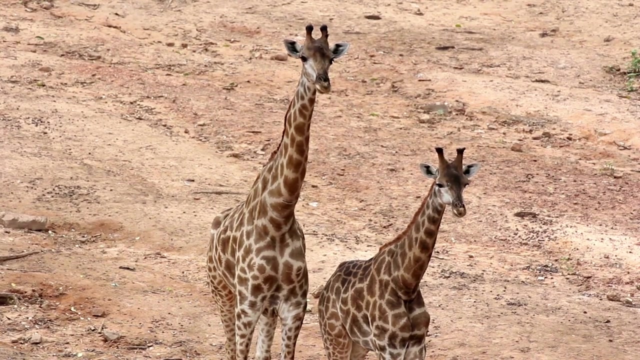 The average height of a female giraffe is 18.5 meters. The baby giraffe gets most of its height in the first three years after its birth. They become adult at the age of four years. If it is male it can get about 18 feet tall, and if it is female then it will get about 14 feet tall. 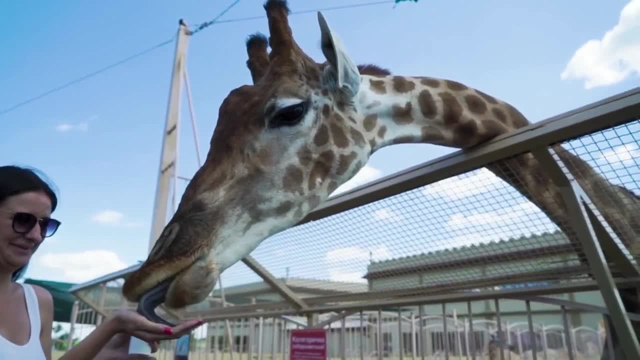 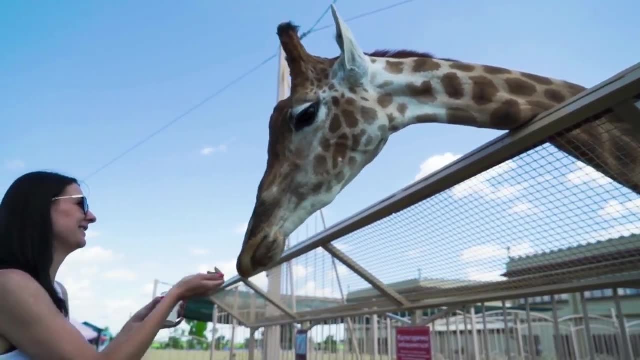 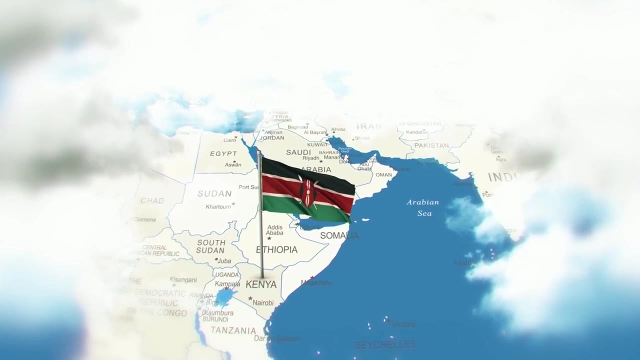 The tallest giraffe in the world ever recorded was about 19 feet tall and was called George in Cheshire, England, back in 1959. It was brought from Kenya and it died in 1969.. Currently the tallest giraffe is Zulu, which is just over 19 feet tall. 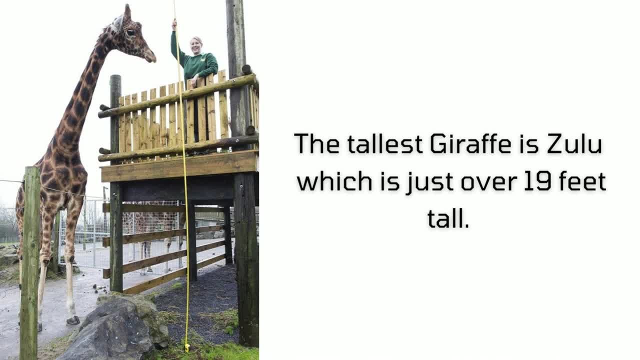 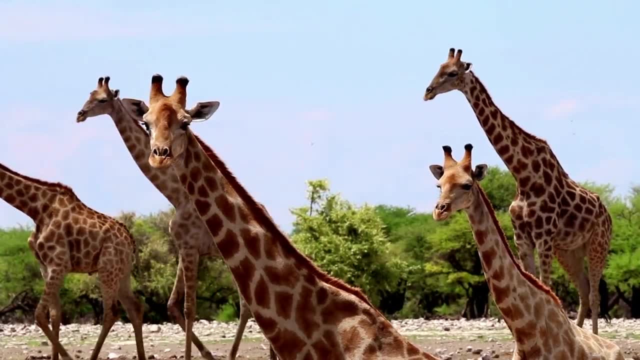 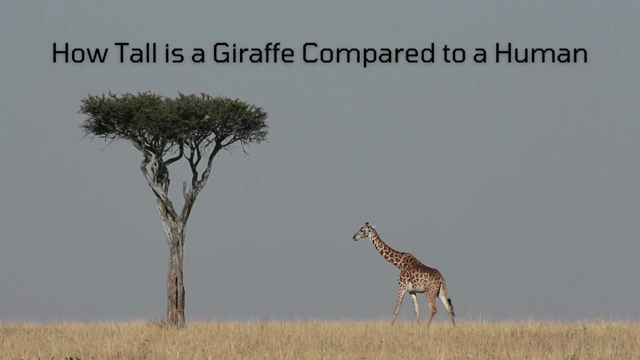 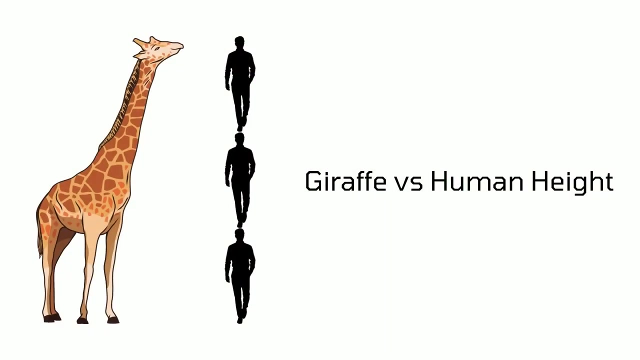 It is kept in Folly Farm Zoo in Saundersfoot and Tenby, Pembrokeshire, England. Zulu is about four feet taller than the average giraffe and is currently the tallest animal in captivity. When compared to human, the giraffe is taller than three adult humans standing on each other's.